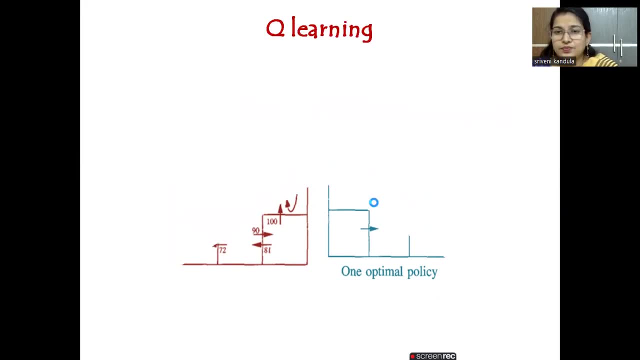 policy with the help of a numerical example. Okay, So before to that, let us see what is meant by Q-learning. So in a Q-learning, it has to acquire optimal control strategies from the delayed rewards, even when the agent has not received a reward. So in a Q-learning, it has to acquire optimal control strategies. 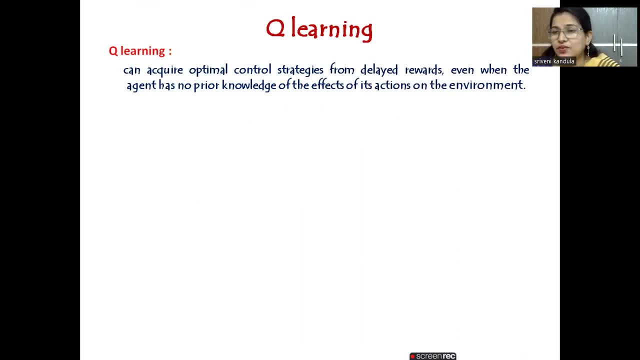 So in a Q-learning it has to acquire optimal control strategies from the delayed rewards. There is no prior knowledge of the effects of its actions on the environment. This is the basic definition that we have seen in the earlier session, right In the reinforcement. 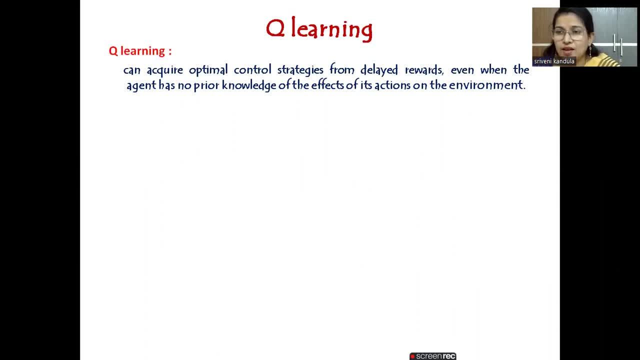 learning. the agent has no idea of the environment, And if he performs a particular action, whether he will receive a reward or a penalty, he is not at all aware. Entirely, he has to do it on a trial and error basis. So now an optimal control strategy has to be developed. 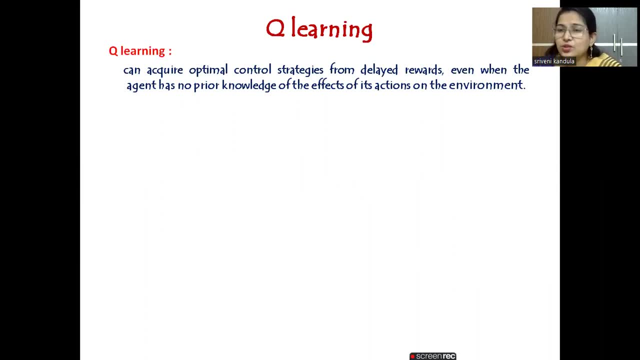 Based on the actions that he is performing. So that is what meant by the Q-learning. So here you can see, we have the agent and he will be performing an action on this environment, And whenever he performs this action either, he will receive a reward. So this reward can. 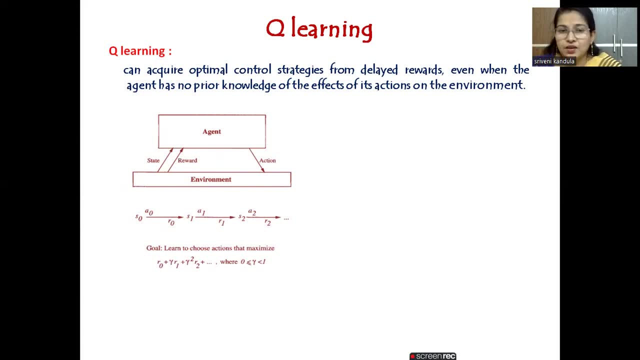 be a positive one, or it can be a negative one, Stated mathematically. here you can see the agent is in state S naught and he will be able to perform an action on this environment. The agent will start performing an action onальныхst joke. 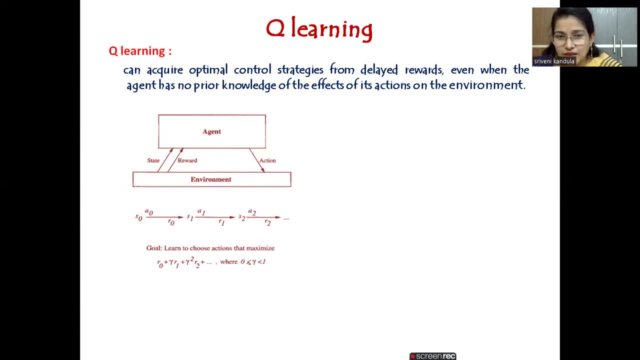 and receives an immediate reward, an additional reward R naught, And this action will lead to a future state S-1, future action a-1 and a future reward r-1.. So like that, whenever he performs a particular action, he will be changing to the another state and 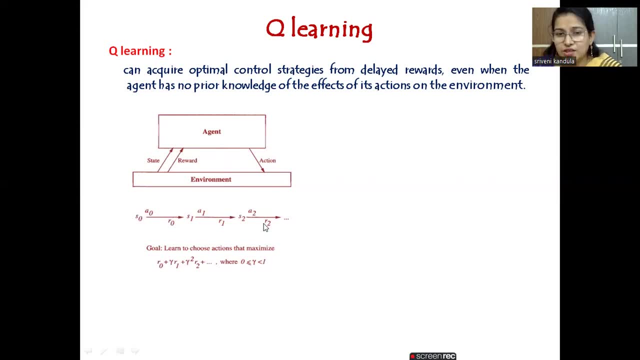 he'll perform. you select the next action and the next reward, So this reward can be a positive one or a negative one. Drive is learn to choose actions which will maximize the rewards. So the reward starting with R0, which is the current reward, plus the future reward gamma, into R1, where gamma is ranging. 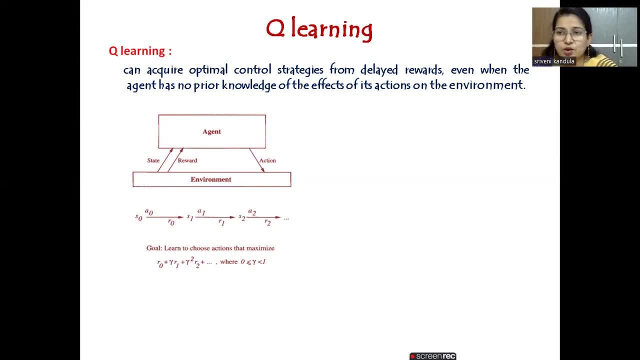 between 0 to 1.. So this is similar to the learning rate, what we have seen, and here this gamma is used as a penalty factor. So here you can see gamma, gamma, square. Suppose if the reward is a negative reward, so then the cumulative reward will be reducing exponentially. 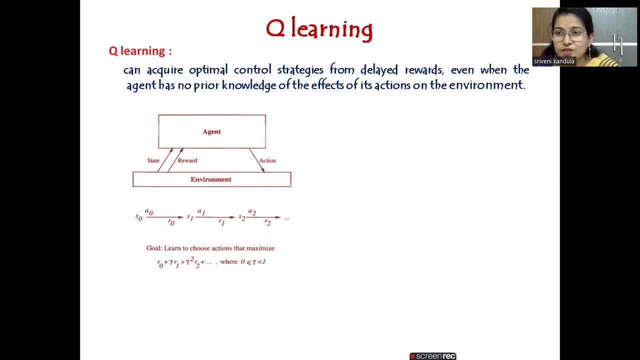 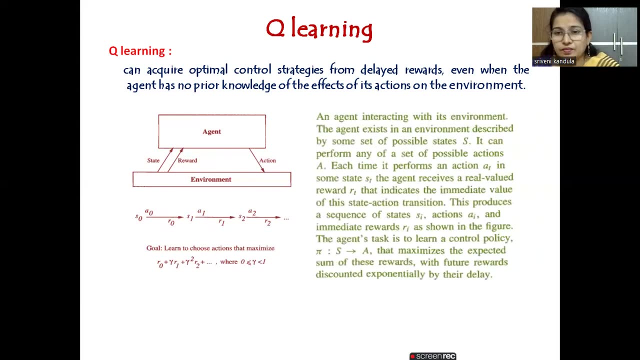 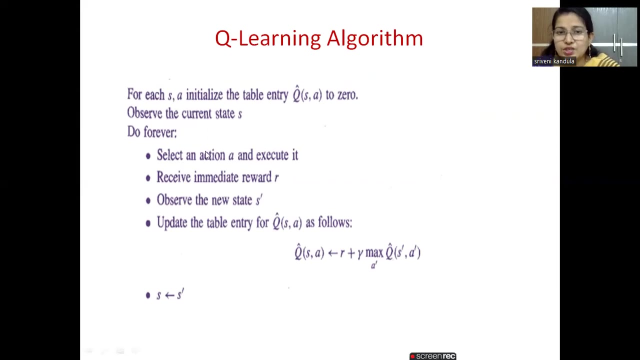 So the agent has to be very careful that he is not receiving the negative reward. always he will receive a positive reward. So here we have the Q-learning algorithm, so which we will be tracing step by step. So, in the initial step, what we have to do is for each 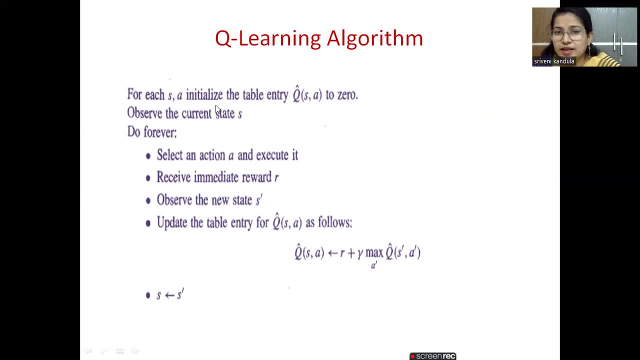 state S and action A. We will be taking a table so that we will be calling as a Q-matrix and that has to be initialized to 0, depending upon the problem that is given. So the number of rows and columns that should be there in the matrix is dependent on the example that we are taking. And then 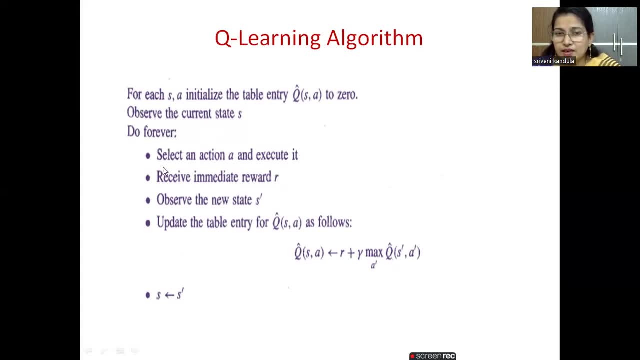 observe the current state and then, repeatedly, you have to perform these steps. What are those? So you have to select an action, execute it and then receive the reward, and then you observe the new state and, based on this new state, update the Q-entry table, So the Q-matrix. 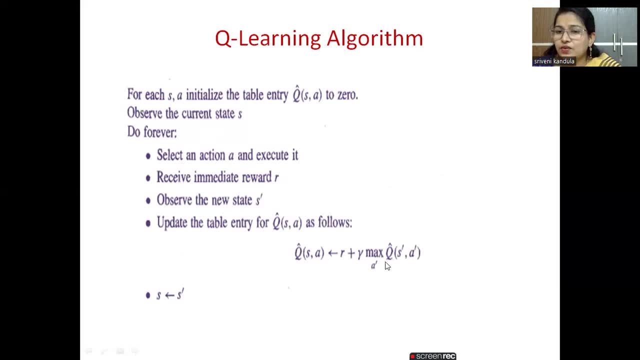 table: whatever is there that has to be updated with the help of this formula, And then the new state, whatever we are having, so that new state will become the current state And with the help of this new state, again iteratively, we have to perform all else. So now let us. 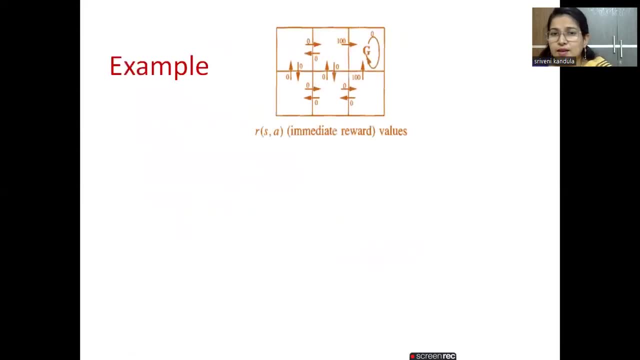 see how to work with this algorithm with the help of a numerical example. So this is the example that is given. So here you can see a maze, So where you have totally six blocks, and in those six blocks, if you just number this, let us number these. 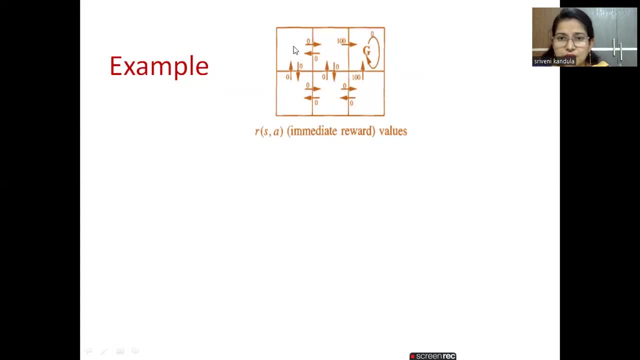 blocks as one. Let us number this. So totally six blocks are there. So you need a Q-matrix of 5, 6 by 6.. And also we will be formulating a reward matrix for the new state. So this is the Q-matrix of 5, 6 by 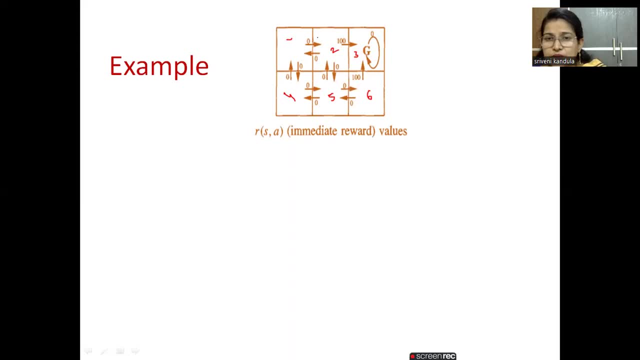 6.. And also we will be formulating a reward matrix for the new state. So here you can see a Q-matrix. So here you can see a Q-matrix of 5,, 6 by 6.. In the reward matrix, So wherever there is no direct path- for example, if you take 1,, 2,, 3, there is. 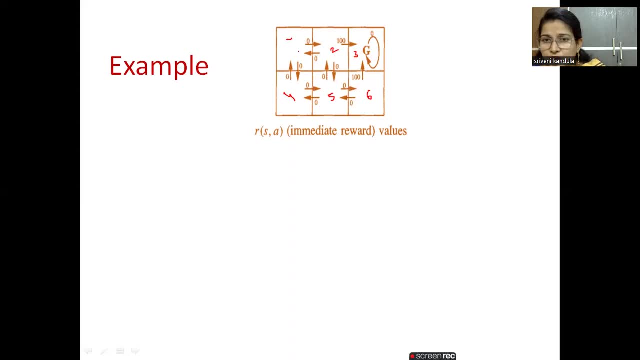 no direct path past rate 2 through 2.. So that is not a direct path. so 1,, 2,, 3 we will be marking as minus 1.. And in all other places we will be marking their reward. that is there. 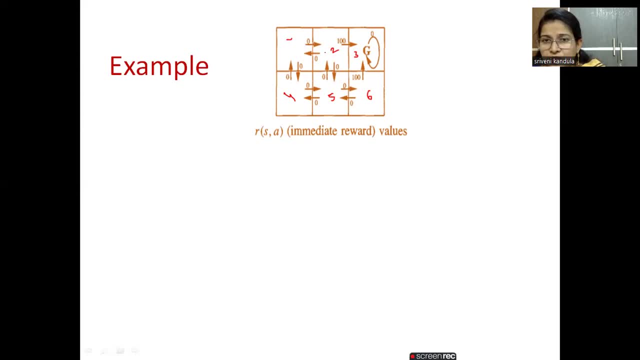 So, for example, if you see 1,, 2, 2,, the reward in 0, and again from 2 to 1, also, the reward is 0, and 2 to 3, the reward is 100.. And from 2 to 5, the reward is 0, and 5 to 2, the reward is 0, and 6 to 3, the reward is 100. 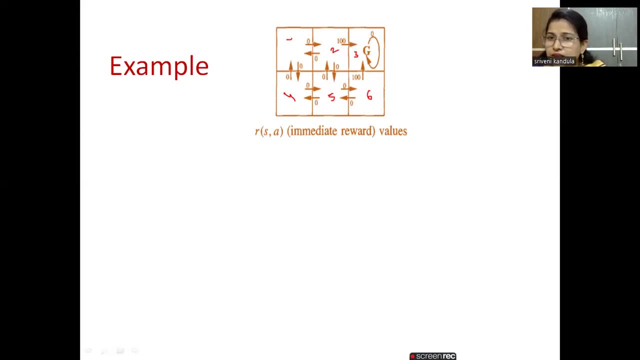 And here one more thing I would like to add on is: so here you can see that 3 means the goal state. So here you can see, there is a self loop with a 0 reward. The reason is: this is an absorbing state. From here we are not going to move anywhere else. 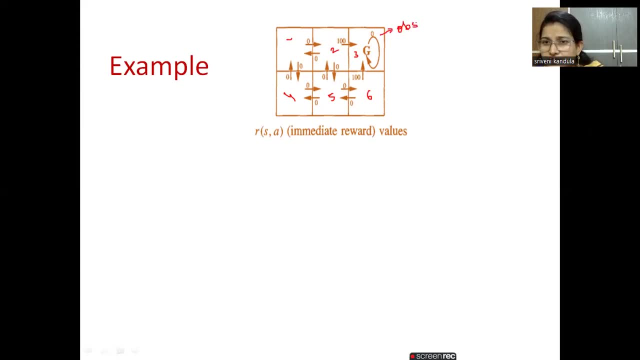 So here the task is learned. This is an absorption state or absorbing state, So it will not have any further reward. So whenever you are giving a self loop to this, you should not give any reward to this. Always the reward will be 0.. 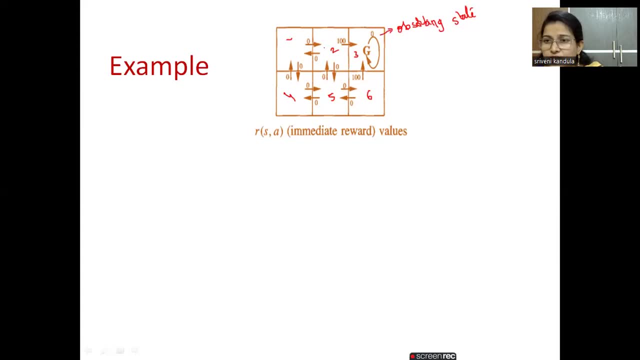 So in other blocks you can give the reward as per your choice, But be careful when you are formulating a new example. this value should not be more than 0. It should not be non-zero. So from this, let us see how to formulate the reward matrix. 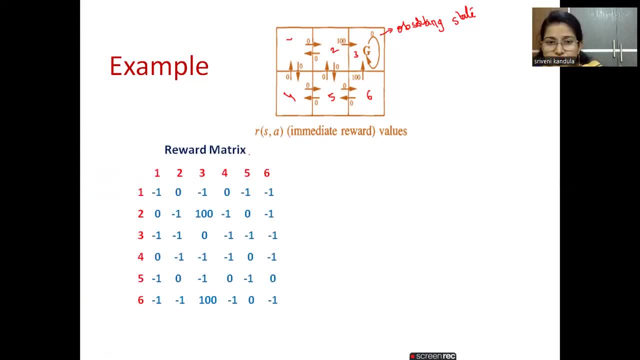 So here I have done the reward matrix for you. So from 2 to 3, the reward is 100.. And from 6 to 3 also, the reward is 100.. And you can see zeros also. From 1 to 2, it is 0.. From 1 to 4, it is 0. 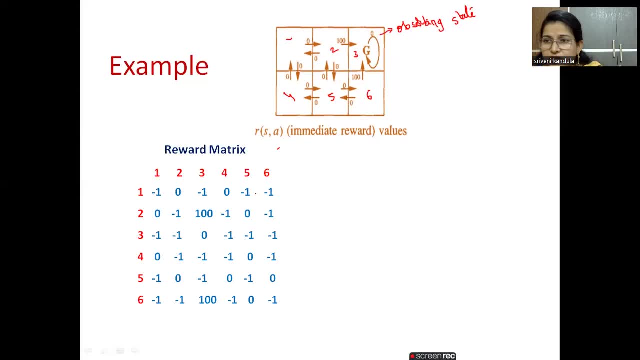 And in all other cases it is minus 1 because there is no direct value. So this is how you need to formulate the reward matrix And similarly, after the algorithm, we have to formulate the new matrix also, In which initially, we will be initializing all sa to 0. 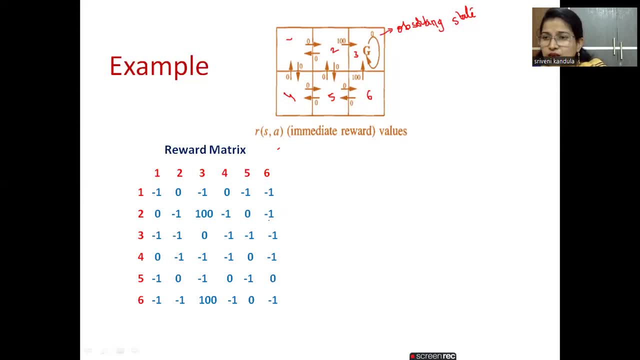 So these are the set of states and these are the set of actions. The rows are the set of states Columns. let us take it as set of actions, So all are initialized to zeros. So now we have to select a state and an action. 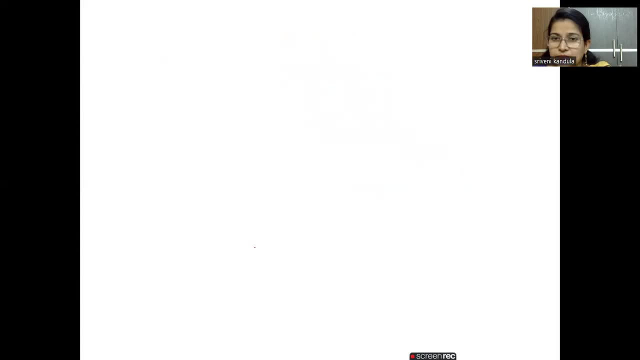 And based on that, we need to move on to the next statement. So which one we have to choose as the beginning. So before going to that, let us see how to obtain an optimal policy. Optimal policy is indicated with 5 star of s. 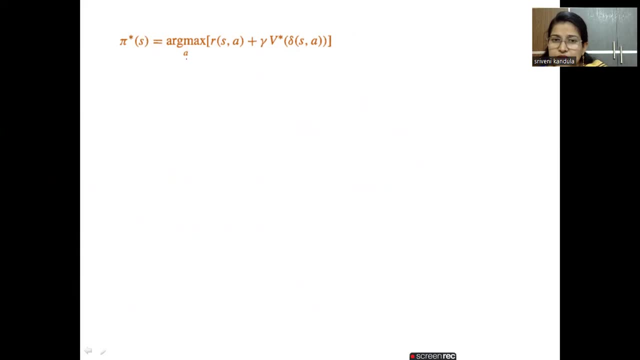 Which is equals to argmax a, which stands for action r of sa plus gamma multiplied with v star of dow of sa. So this is the transition: when you are performing an action in this particular state, You will be moving to the next statement. 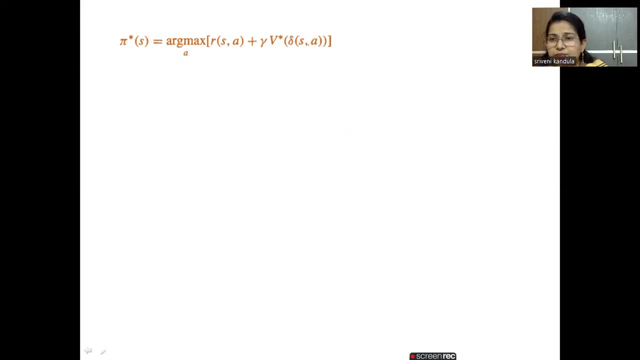 And you will have the next action also. So which, in short, can be written as rmax of a q of sa. So this whole thing, we are taking it as q of sa And to obtain this formula. So in the algorithm we have this step. 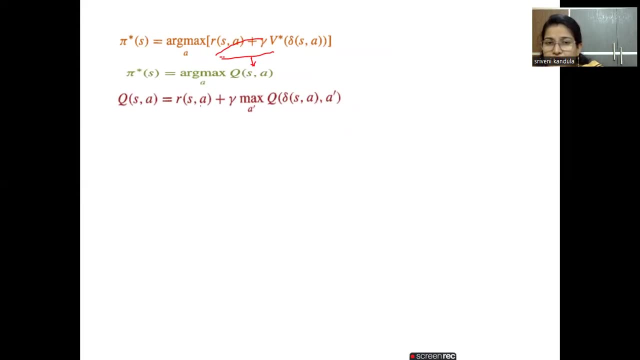 So to update this, we use the formula r of sa plus gamma max a, dash q of dow of sa. You will be moving on to a new state And you will perform a new action, receiving a new result. So for your convenience, I am just giving the reward matrix here. 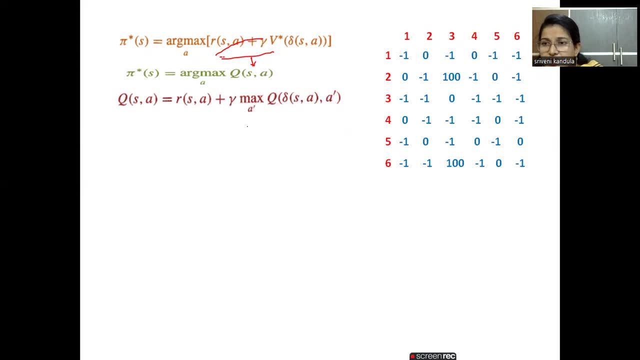 So now here, if you see, 3 is our goal state. So from 3 we cannot move anywhere. So q of 3 comma 3 is 0. So here, randomly, you can select any state of your choice. Okay, So I am starting with 2.. 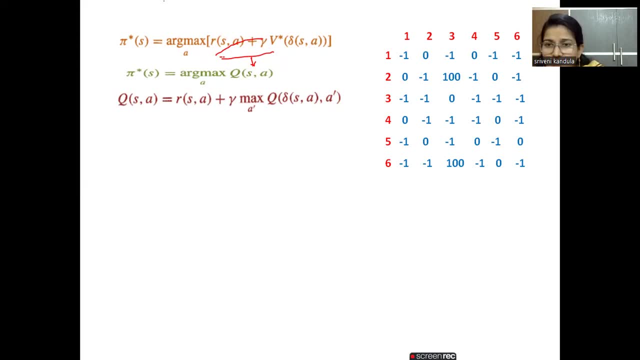 Okay, So in 2.. So that is, let us take the second row. So in second row, what are the non-negative values that we have? So we have 2,1,2,3 and 2,5, right? So 2,1 is 0.. 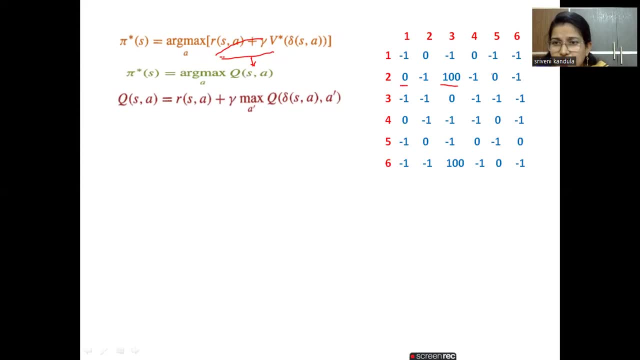 2,1 is 0.. 2,3 is 100.. 2,5 is 0.. So these values we need to first find out And based on that, And based on that we start solving the further ones. Okay. 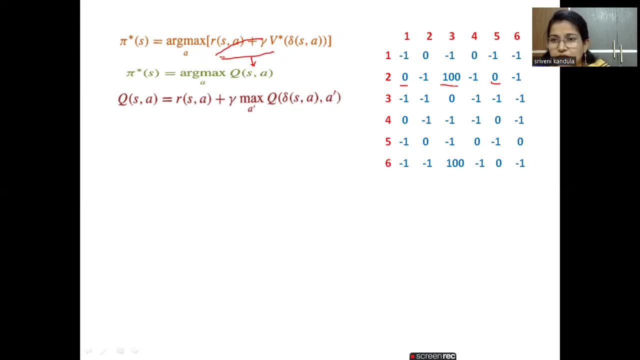 So, since I see a maximum value in 2,3, I start with this value. You can start with any state randomly. You can start with any row of your choice. Okay, So I am starting with q of 2 comma 3.. 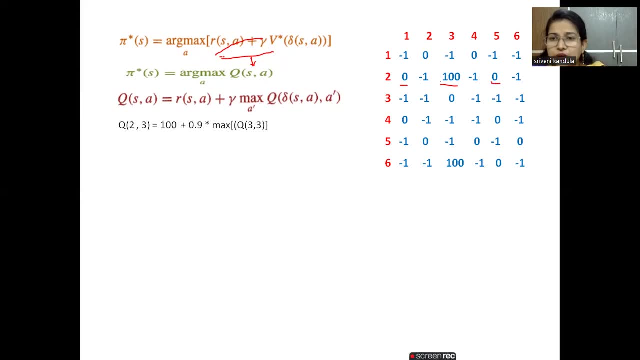 Okay So, which is r of s comma 8.. So here the reward of 2 comma 3 is 100.. Plus gamma value, which is taken as a value between 0 to 90.. Okay, Here it is taken as 0.9 for this problem. 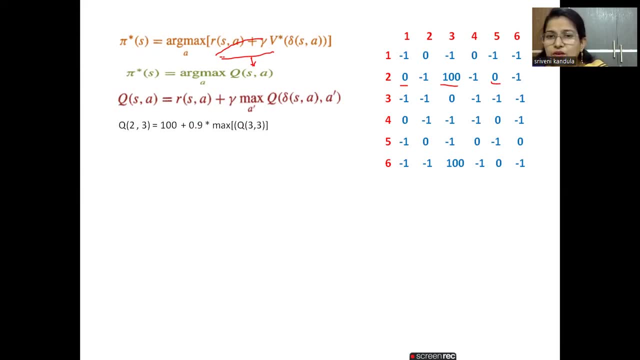 Okay, And max of q of 2 comma a dash. So here from 3.. Okay, So 3 is our new state. So let us go to 3 and let us see what are the non-negative values. So we have a non-negative only in 3 comma 3.. 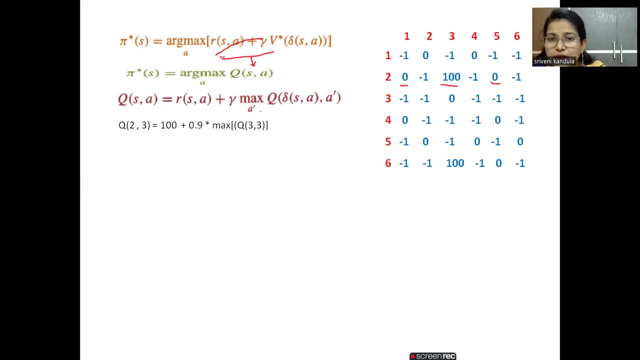 So we will take this: Okay, And the q value for this from the q matrix is 0.. So let us substitute it 100 plus 0.9.. Q of 3 comma 3 value is 0.. This I am taking from the q matrix, not from the reward matrix. 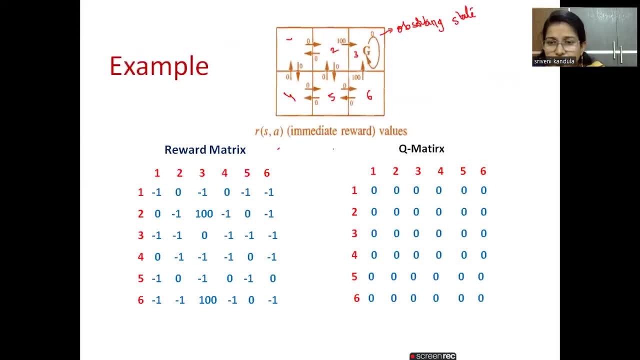 Once I will go back and show you the q matrix. So here the q matrix is initially 0 for all the values. So here I am taking the value 3 comma 3.. So this q value I have substituted. Okay, So reward you have to take from the reward matrix. 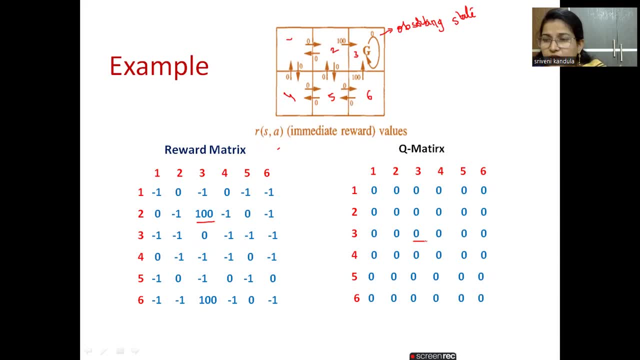 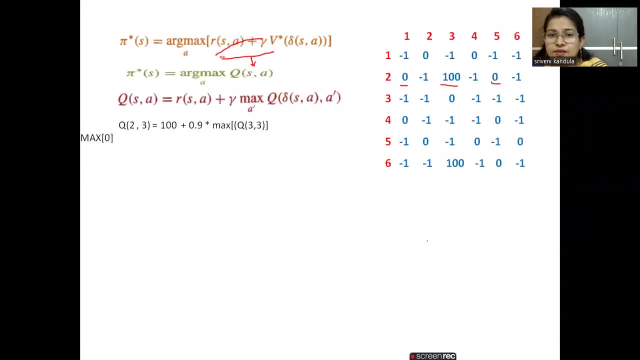 Reward of 2 comma 3, we have taken, And q of 3 comma 3, we have taken. This you should be clear. Then it is very easy to solve this problem. Okay, So now, since I am seeing one more maximum value in 6, the next row I am selecting. 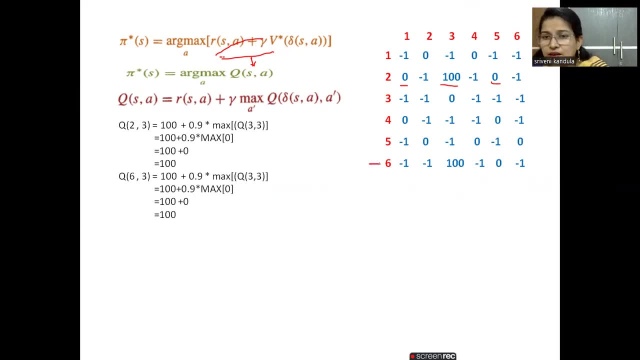 This is the next iteration, So 1 is done, So I am randomly selecting 6.. So here, q of 6 comma 3 is again r of l, Which is r of 6 comma 3.. The reward value is 100.. 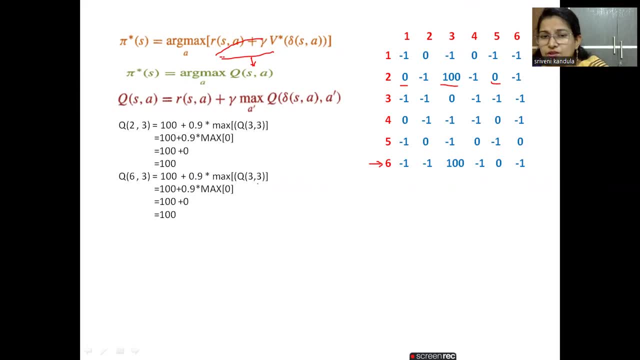 Plus 0.9 into max of q of 3 comma 3.. And if you solve this you are obtaining a value of 100 comma 100.. Let us update our q matrix now. So here you can see I have updated the q matrix. 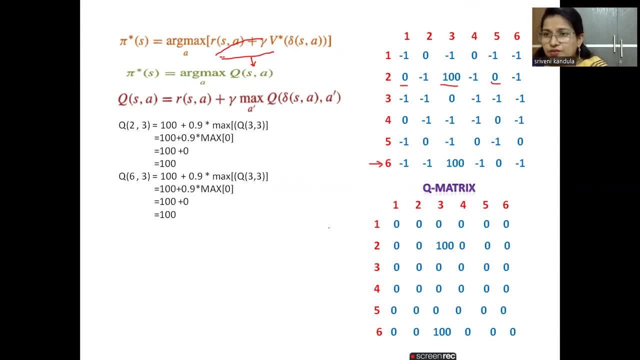 And let us proceed further. So let us do more and more iterations in order to update the other values. So next, I have selected randomly the first row. So in the first row the non-zero values are in 1, 2 and 1, 4.. 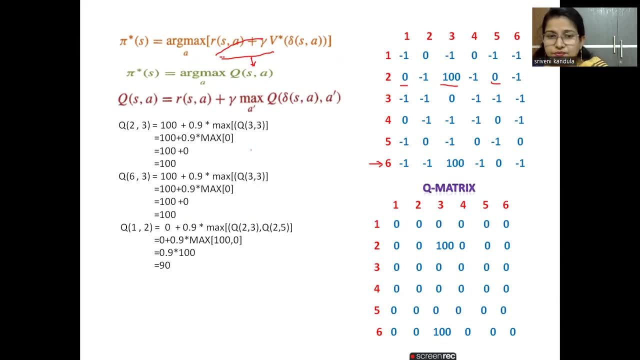 So first, I am solving for 1, 2.. Okay, So the value that we have obtained is 90. And 1, 2, whenever you are selecting The next state, is always based on the action that you are taking. So action is 2.. 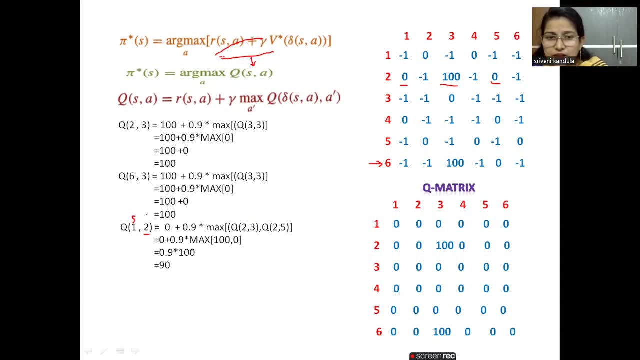 This is s comma, a right. The first value is s, The second one is a, So whenever you are performing the action, a, So this 2 is selected as the next state. So, with the 2, what are the possible transitions that we are seeing? 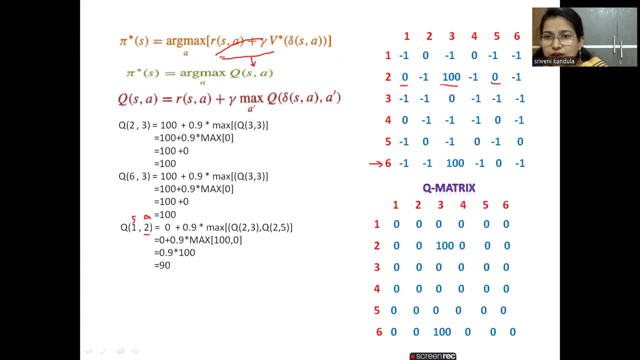 So from 2, where can I move? I can move on to 2, 1.. I can move on to 2, 3.. I can move on to 2, 5.. So these are the possibilities. So here, 2, 3,, 2, 5.. 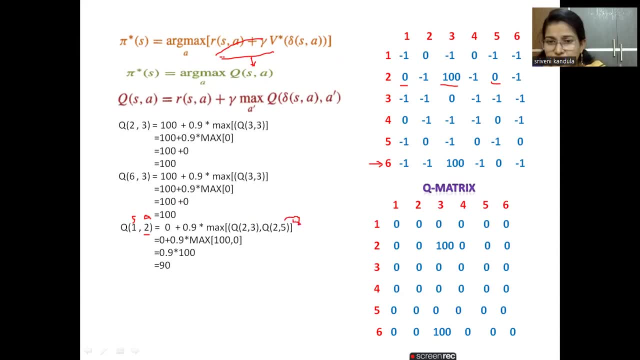 I forgot to add on 2, 1.. So we just add that also. 2 of 2, 1 also to be added, Which is anyhow 0.. q value of 2, 1 is 0.. q value of 2, 3 is 100. 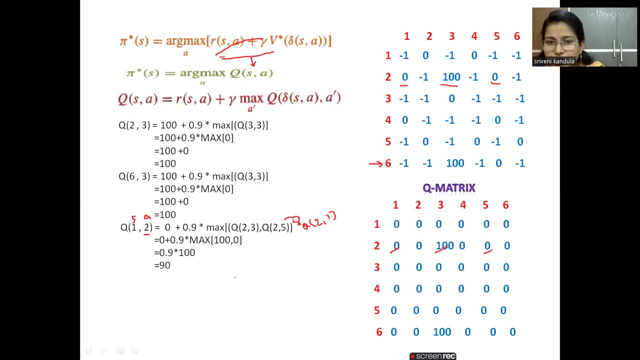 q value of 2, 5 is 0.. So it is 100 comma 0 comma 0.. So maximum value of this is 100.. 100 multiplied with 0.9 gives us a 92.. So this has to be again updated in the q matrix. 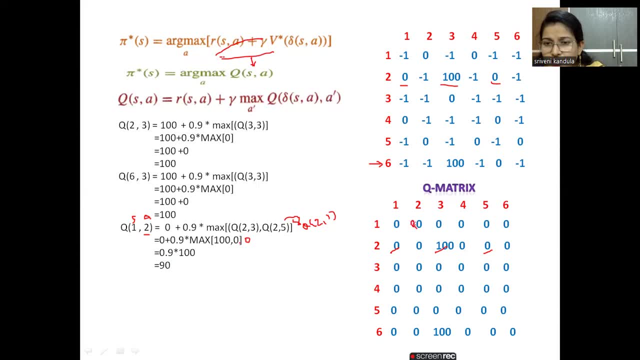 Where you have to update, You have to update here in 1, 2.. So 1, 2 will become 19.. For the next iteration you have to take these updated values. So now the control policy is updated Step by step iteratively. 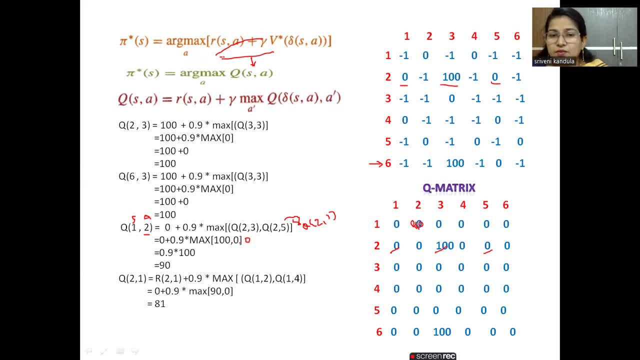 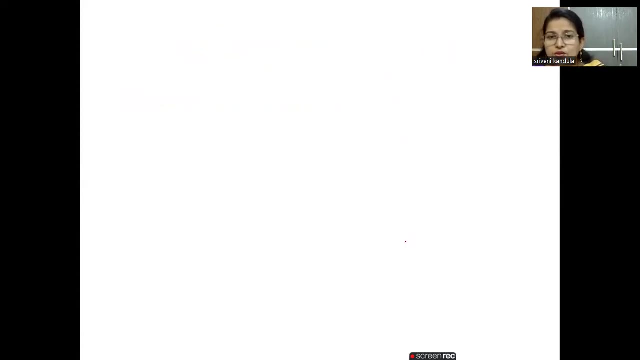 Again we are finding 2, 1.. The value that we got is 81. Let us update these two. So here in 2, 1 you have to update the value to 81. So, similarly, all other values you can just find out. 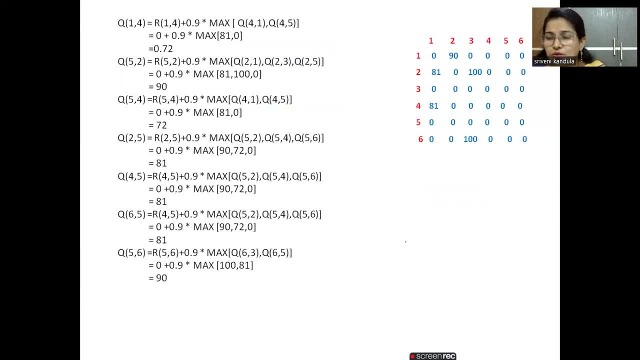 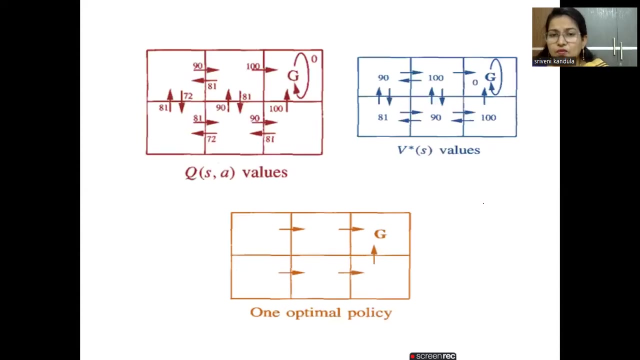 I have just listed out. You can work on this on your own And the final q table that is updated also, I am giving for you all. So this is the final updated q table that we are obtaining And based on this you have to formulate q of s comma values. 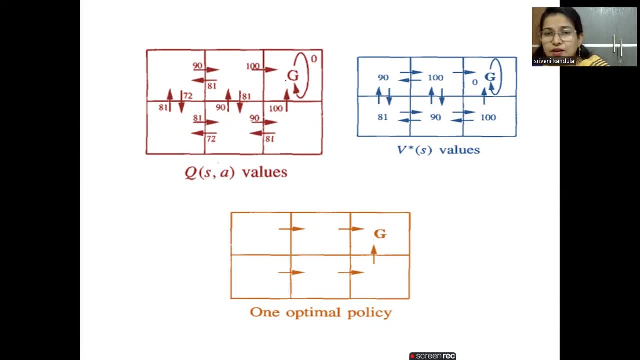 So this is the initial one that is given. So initially the values are 0. So now we have updated, So the agent has updated all its values. So these are the updated values. Out of this, what we have to select. We have seen that it should be an argmax. 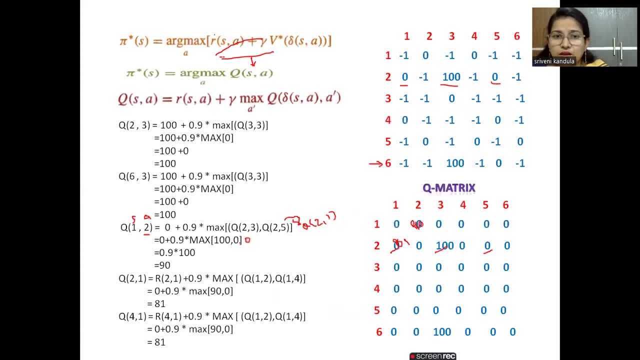 I will just show you that 5 star of s is argmax of a, q of s, comma a. So wherever these q values are maximum, You know how to use the argmax. So maximum value of the available ones we have to pick on. 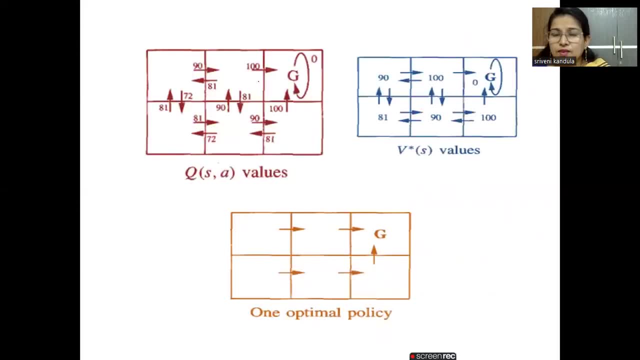 So, based on that from here, So now in this particular block, if you see So here you have a value of 81, comma 92.. Only the incoming arrows I am considering, Ok, Incoming, or leaving. So among 81, 72, 90 and 81, the maximum is 90.. 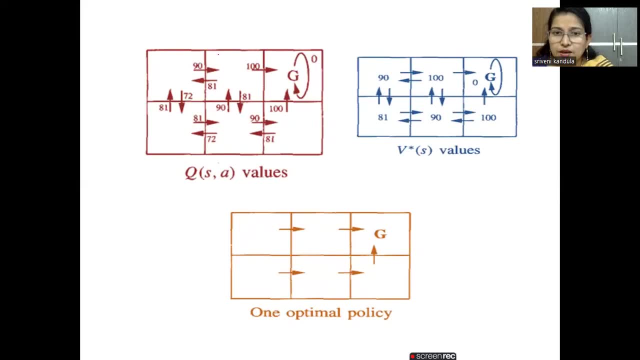 So max value we have to consider So 90.. So here in this particular one, the maximum value is 100.. So here in this in 4, the maximum value is 81.. So here in 5, the maximum value is 90.. 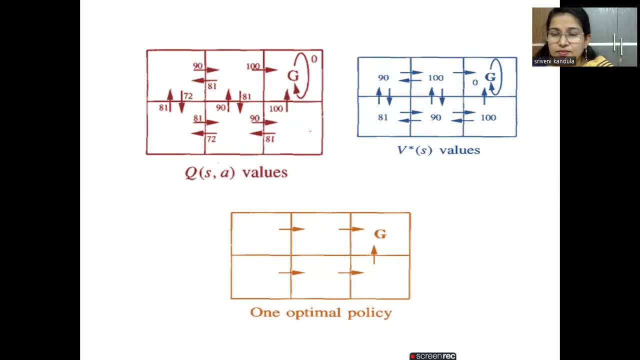 So that we are picking In 6. the maximum value is 100.. So that we are picking And the optimal control policy that we can give is Always our aim is move towards the goal. So either the agent can start with 1.. 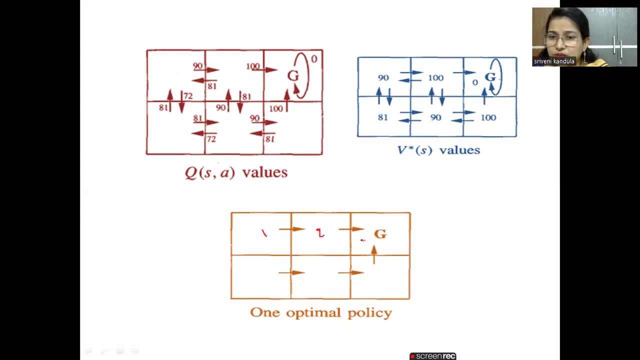 Ok, So start with 1, move to 2 and then to 3.. Or he can start with 4. And then move from 4 to 5 and then to 6.. Ok, So this is one control policy that we can do.